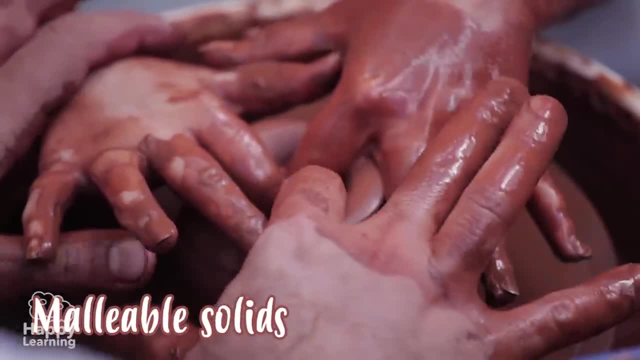 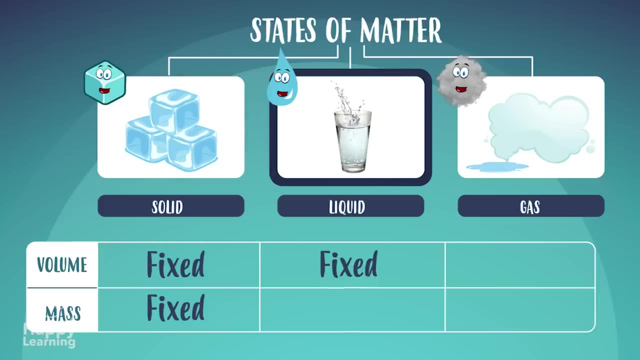 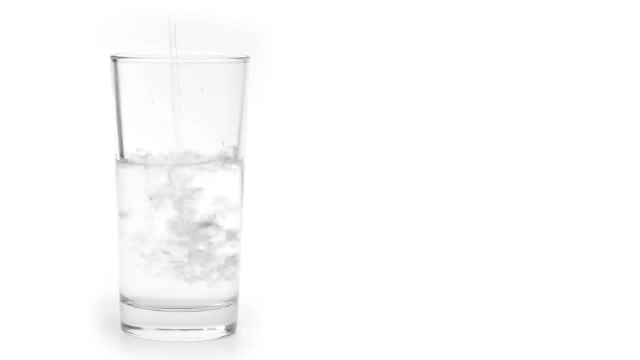 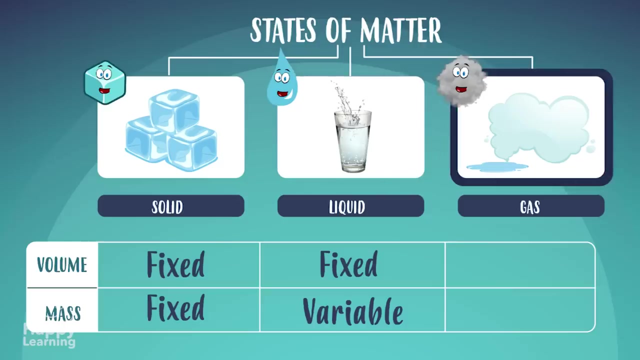 In these cases, they are malleable. solids- Liquid state- is characterised by having a fixed volume and variable size. Liquids take the container's shape, like this glass or jug. Gas state is characterised by having a variable volume and size. 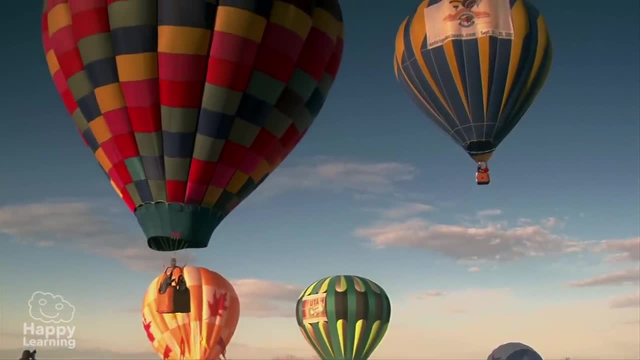 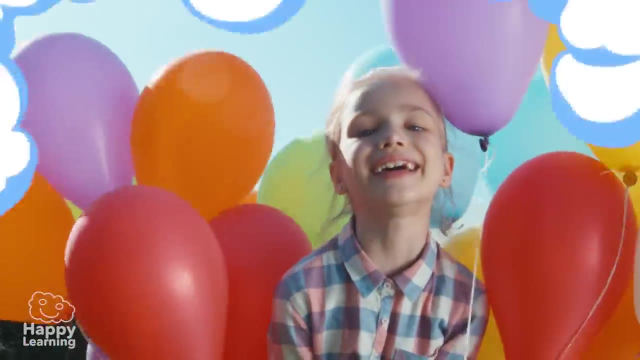 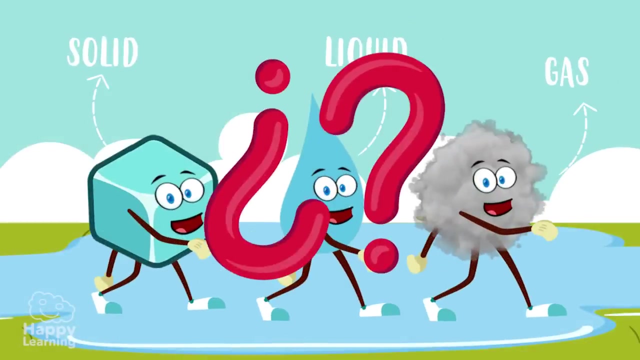 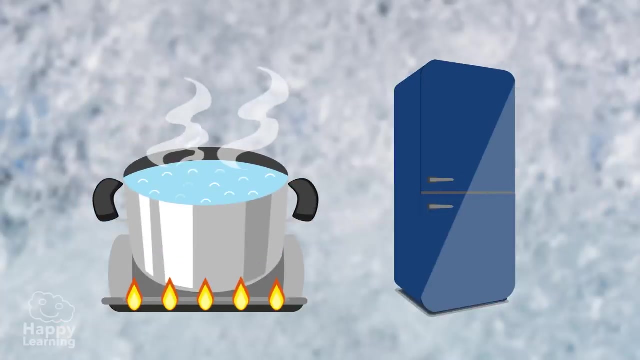 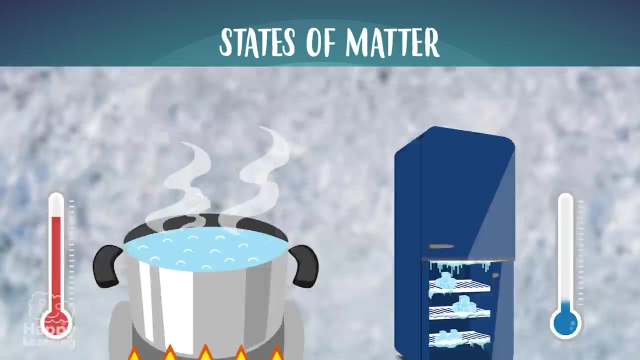 In the same way that liquids take the shape of the container holding them, but gases always occupy the full volume of the container. Now we know about the three states of matter, but do you know how we can change from one state to another? Changes in state happen after cooling or heating matter, and there are different types. 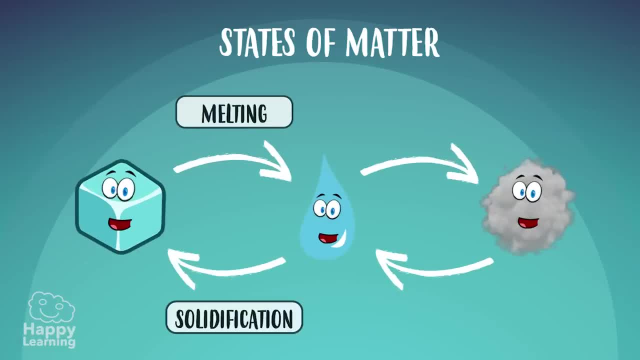 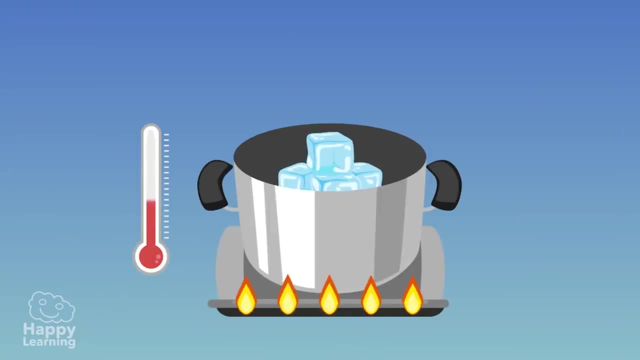 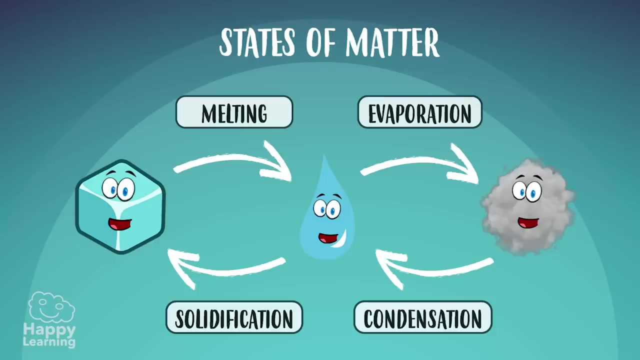 Melting, solidification, evaporation and condensation. Melting happens when matter changes from its solid to liquid form and happens after rising temperature. When we heat an ice cube or leave it at room temperature, it melts And changes from solid to liquid. 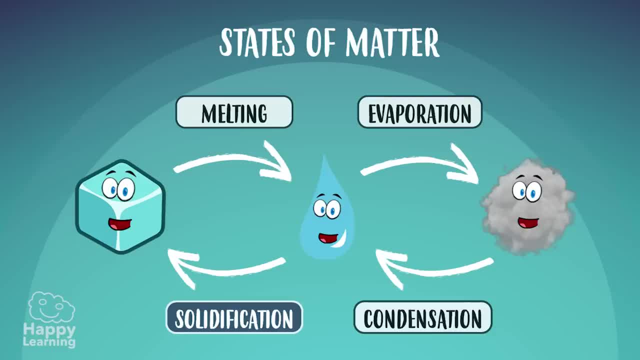 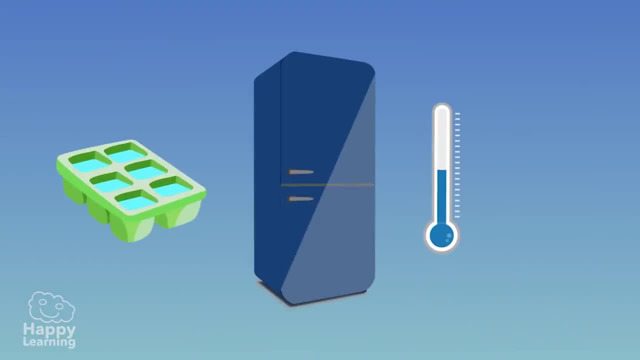 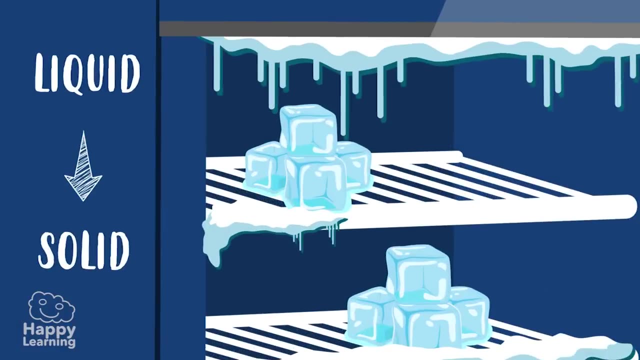 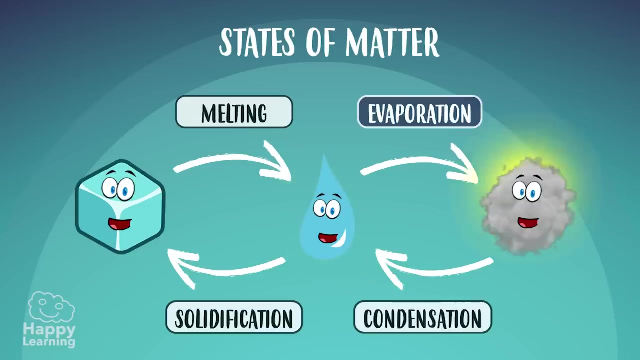 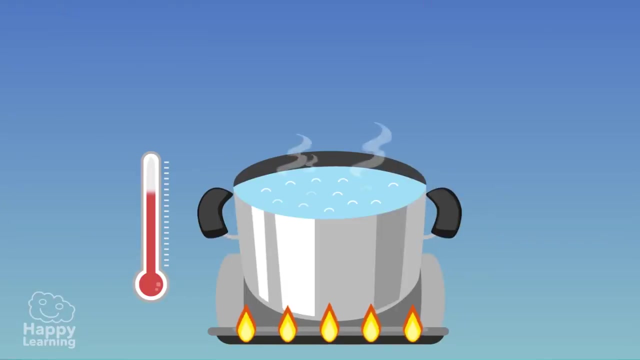 Solidification is the opposite from melting. Matter changes from liquid to solid form. It happens when we put water in the freezer and it turns into ice. It goes from liquid to solid. Evaporation is when matter changes from liquid to gas After liquids are heated. for example, when we boil water, it turns into water vapour. 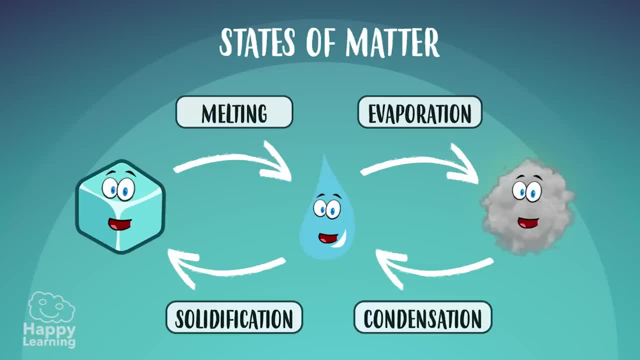 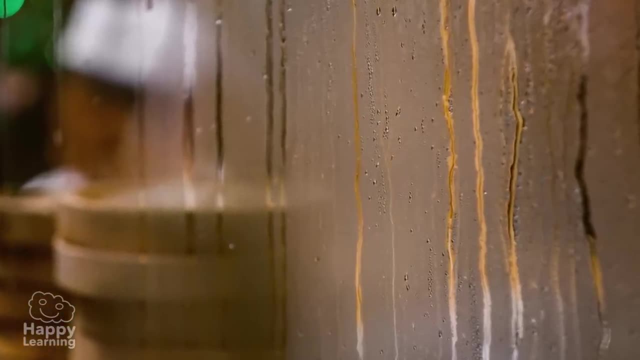 It turns from liquid to gas. Condensation is a step from gas to liquid and happens when matter in gas state is cooled. Have you ever noticed that when we get steamy windows or mirrors, water droplets appear? It's produced when water vapour turns into steam. 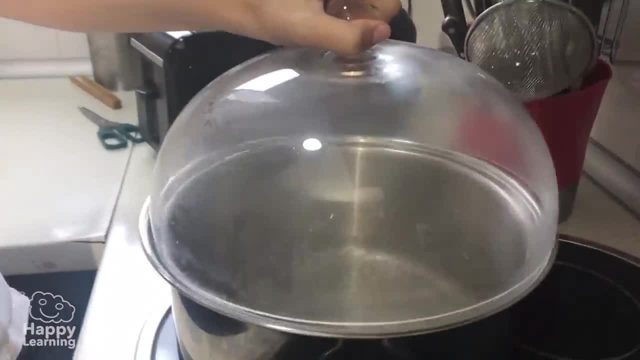 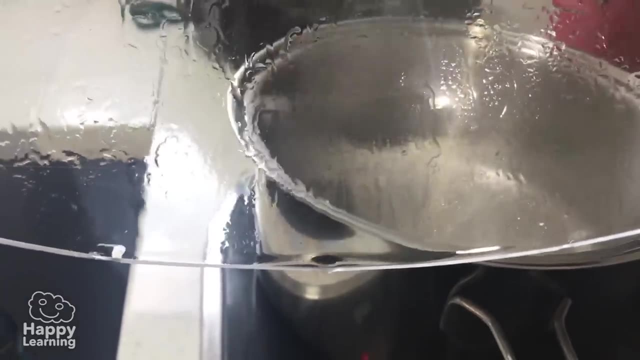 It's produced when water vapour turns into steam. It's produced when water vapour turns into steam. It's produced when water vapour touches a cold surface. In that same moment, water vapour cools and turns into liquid. Easy huh. 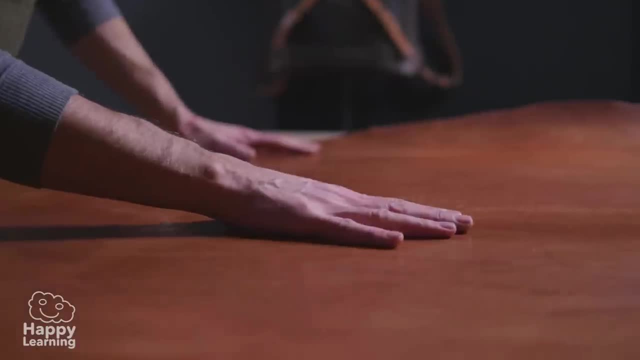 Well, now we know the states of matter. Goodbye friends, and don't forget to subscribe to Happy Learning TV.